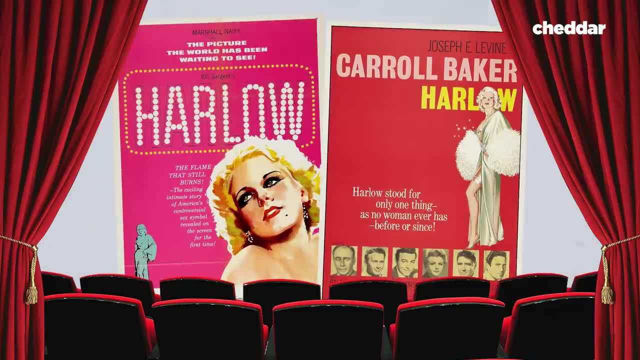 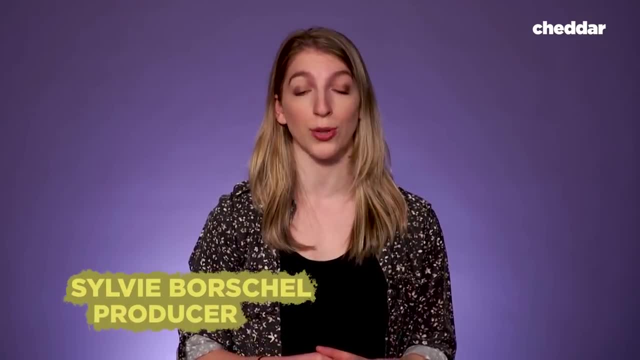 Harlow, which didn't even bother to come up with different names for the films about actress Jean Harlow. And this was just the start to what would eventually become an extremely common occurrence throughout cinematic history. As is with most twin films, one of them usually does really well at the 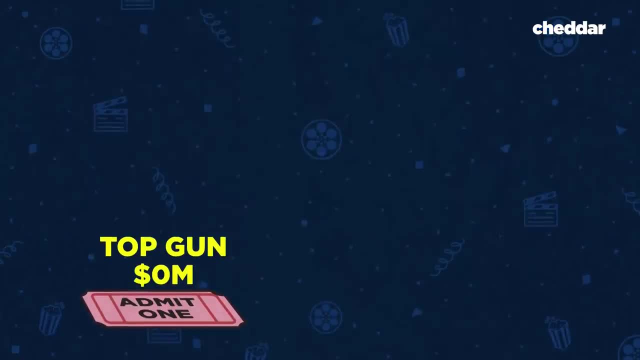 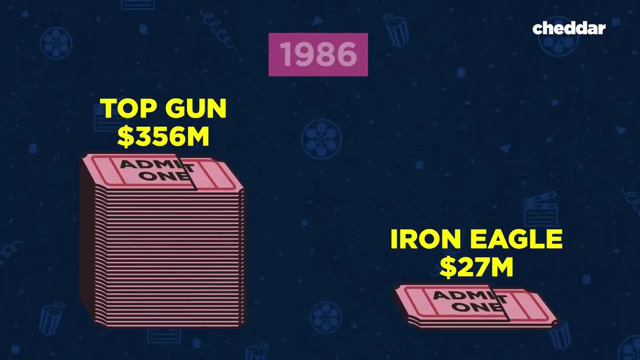 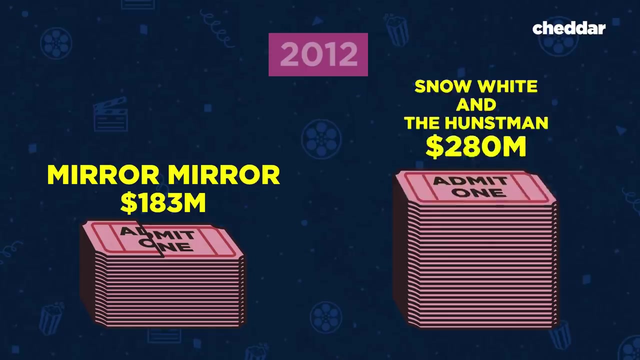 box office, while the other one doesn't. Take Top Gun and Iron Eagle for example. Both were released in 1986, but Top Gun beat out Iron Eagle by a landslide, despite Iron Eagle being released first In 2012,. Mirror Mirror couldn't compete with Snow White and the Huntsman. 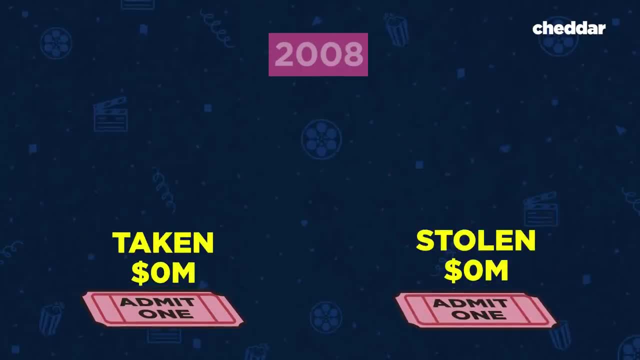 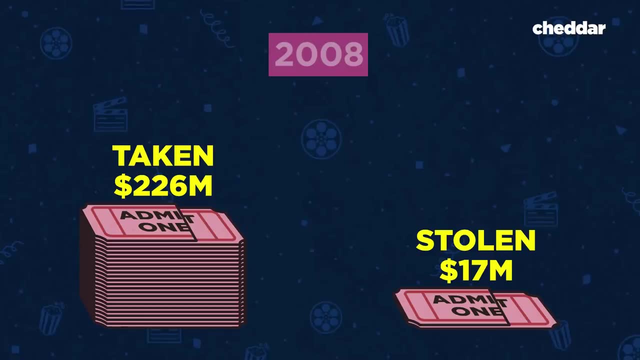 With Taken and Stolen. their similarities ended after having the same plot and being released in the same year. One of them tanked at the box office while the other one soared and is still being quoted today. But what I do have are a very particular set of skills. But if there's no, 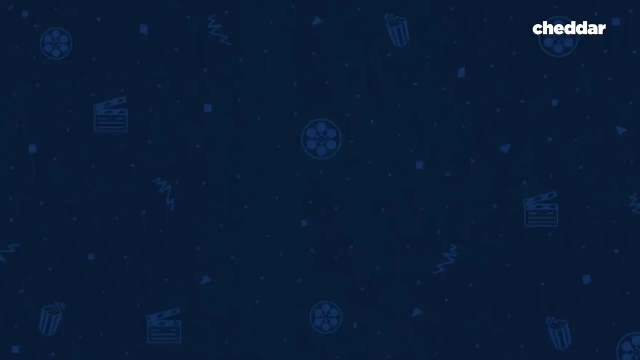 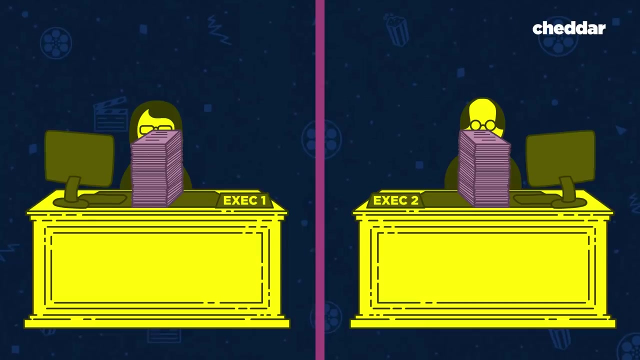 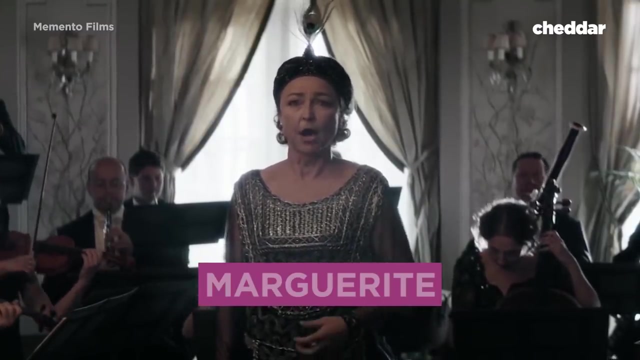 guaranteed success. then why do twin films happen? Well, sometimes it's just plain coincidence: Two scripts about the same film just happened to pop up on desks of two different studios around the same time. Take the 2015 film Marguerite, which was based on socialite Florence Foster Jenkins. 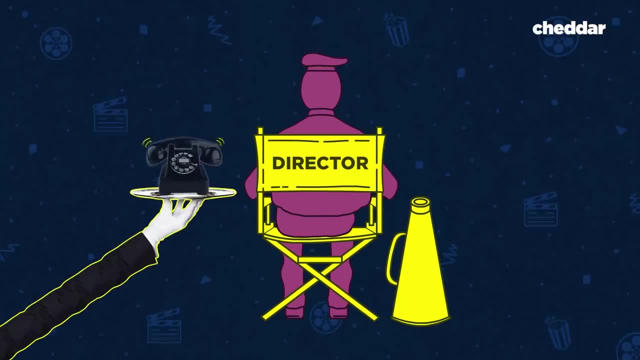 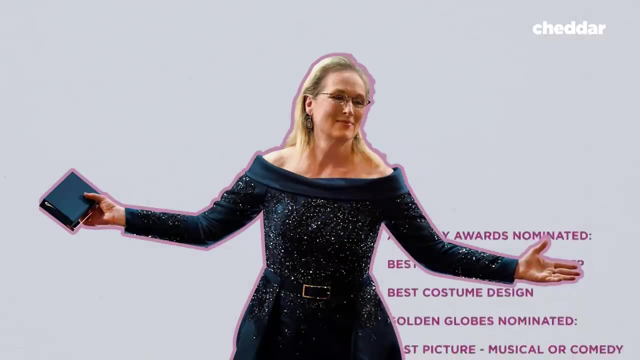 The director found out about the competing film titled Florence Foster Jenkins starring Meryl Streep one month before he started filming, and he knew his film was done. The latter was widely praised during the awards season that year, But in other cases some films might be inspired by the same. 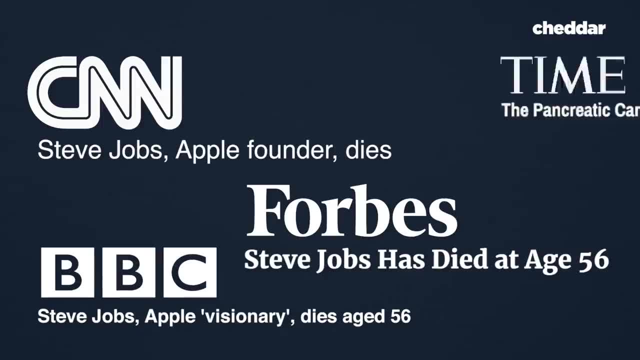 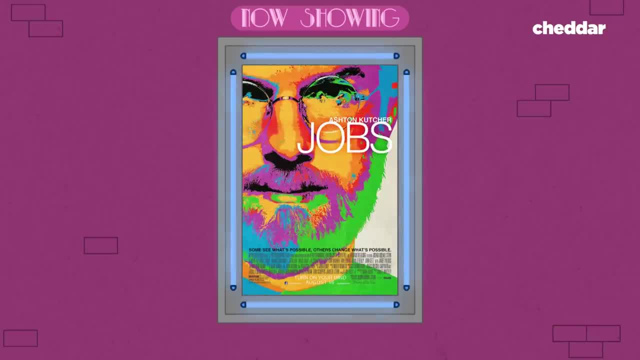 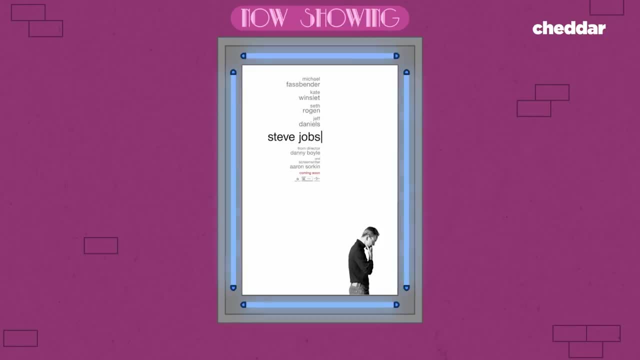 or tragedy around the same time. After the passing of Apple co-founder Steve Jobs in 2011,, two screenwriters began developing films around his life and death. Jobs starring Ashton Kutcher was released first in 2013 as a bit of a flop, while the other film, Steve Jobs, took its time. 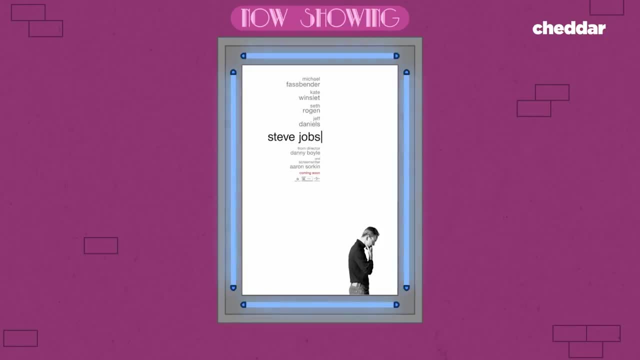 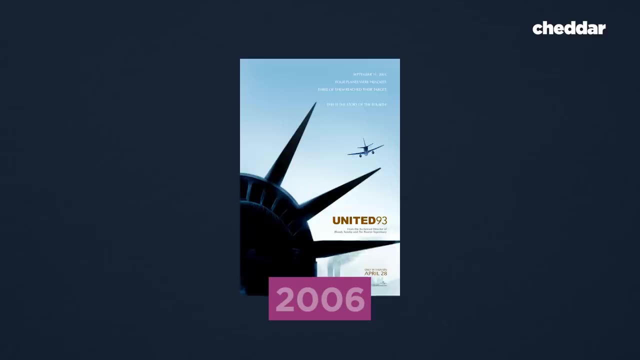 during the writing and development stages and was finally released in 2015, to great success, And five years after the tragedy of 9-11,, 2006 saw the release of United 93,, Flight 93, and The Last of Us. The film was released in 2013, and was released in 2015.. 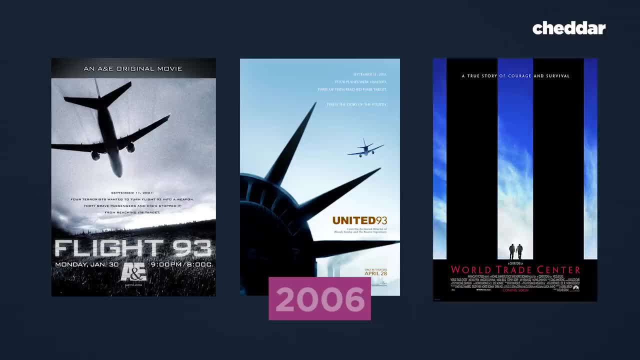 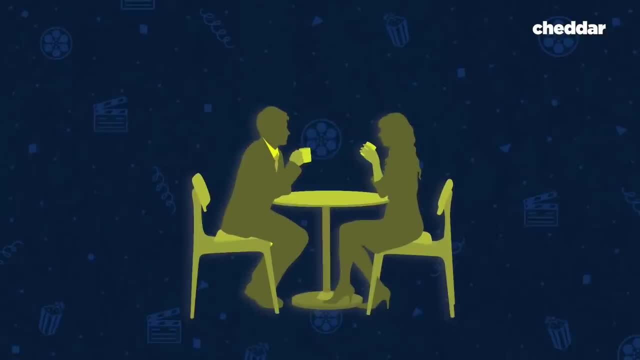 The film was released in 2013, and was released in 2015,. and was released in 2015.. and Nicholas Cage's World Trade Center, all inspired by the events of 9-11 and all released within months of each other. Other times, though, it's far from coincidence, A studio might hear. 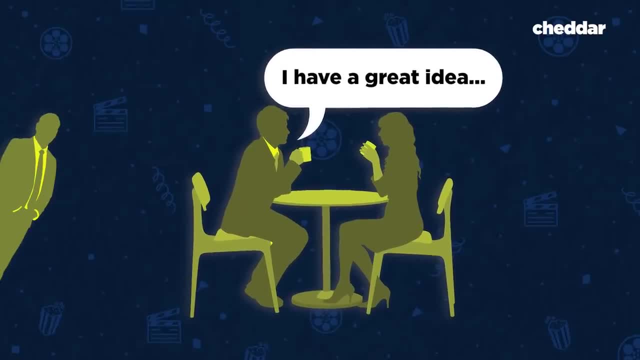 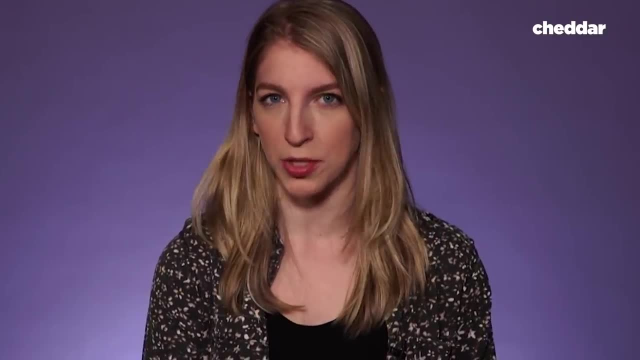 of another studio having a great idea, love it, steal it and try to make it better and faster. While not everybody has come out and admitted that- because who's going to admit to plagiarism? these films have enough evidence to support the drama that supposedly played out underneath the 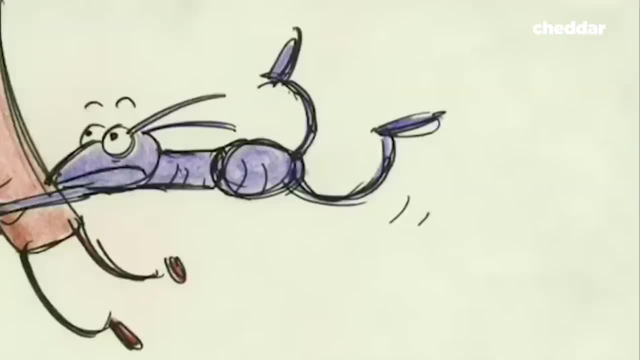 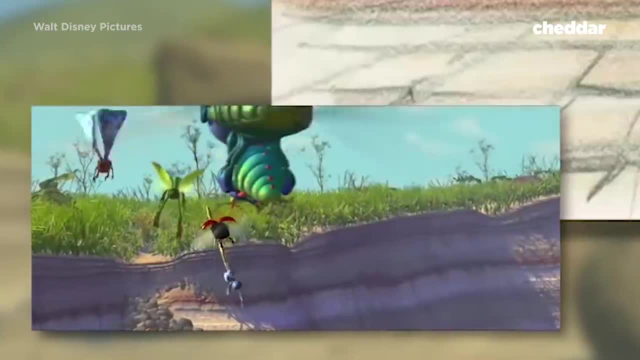 surface. Ants vs A Bug's Life. Ants vs A Bug's Life. In 1988, Disney pitched a story about army ants which would later become A Bug's Life, But after a feud with Disney's CEO, Jeffrey Katzenberg left the company. 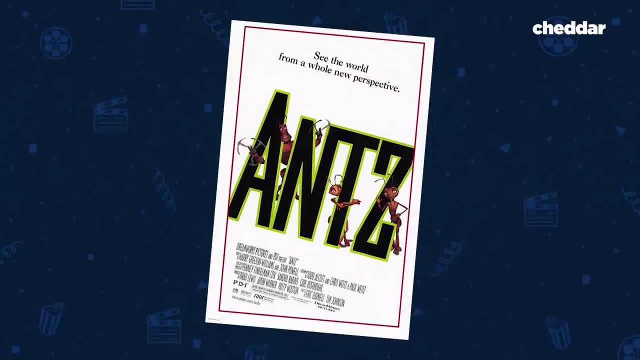 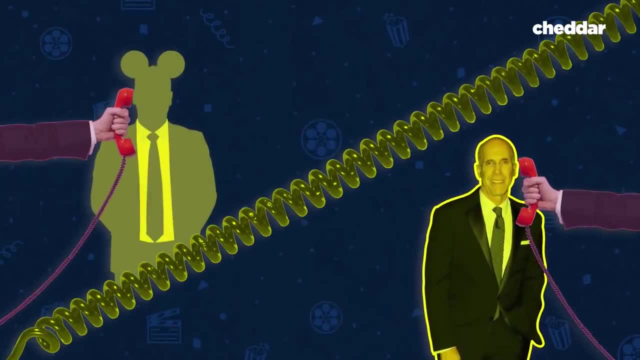 took the story and brought it to Dreamworks, And so Ants was born. The speculation on the story being stolen had gotten so big that a Disney executive had called Katzenberg himself to ask him if it was true, And Katzenberg confirmed it. 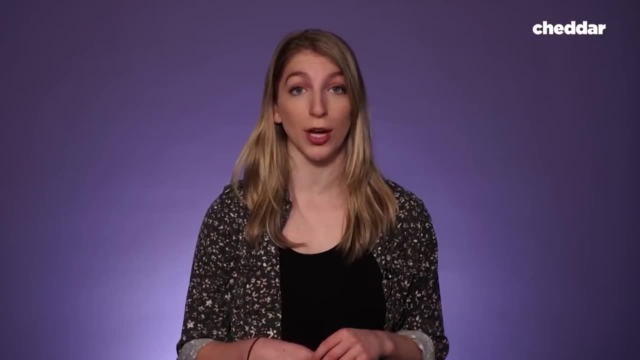 There were even rumors that Katzenberg bribed Disney to slow down the production of A Bug's Life, and if he did, they would halt the production of Ants. Well, it looks like that didn't exactly work out in his favor. 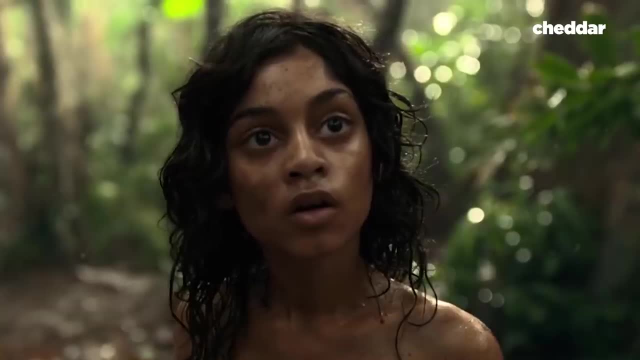 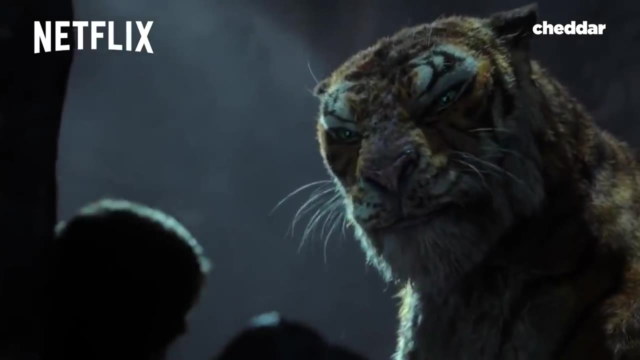 Mowgli vs The Jungle Book. We recently saw the release of Mowgli, the live-action Jungle Book film on Netflix. It felt all too familiar because in 2016, we saw the release of a different live-action Jungle Book film titled well, The Jungle Book. 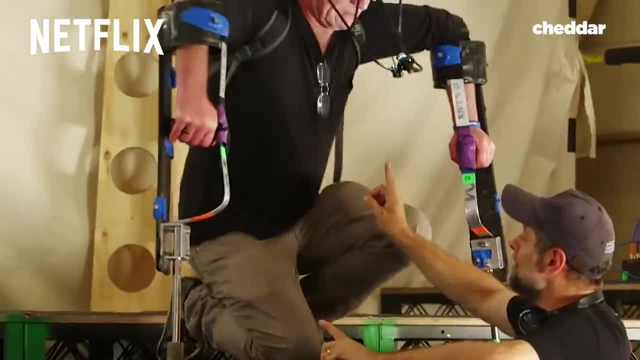 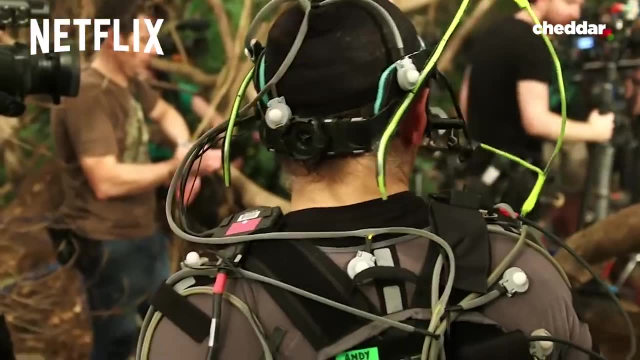 The Warner Bros film Mowgli had actually started production first in 2012 and was scheduled to be released in October of this year. The movie has been released for the first time since the first release in October of 2016.. And shortly afterwards, Walt Disney Pictures happened to. 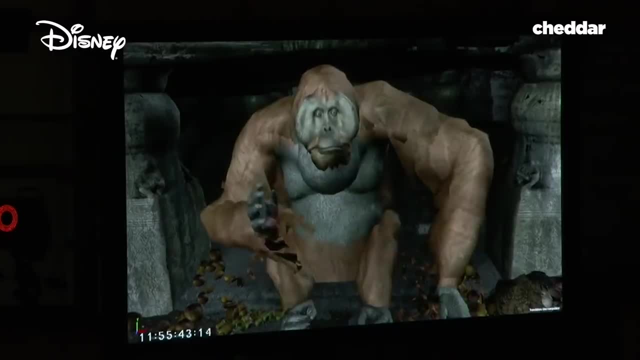 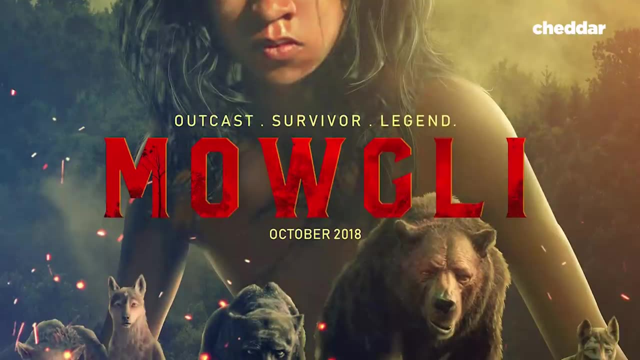 also announce that they were making a live-action adaptation of the story, but that they would be releasing the film in April of 2016,, conveniently before Mowgli was set to be released. Mowgli ended up pushing their release date to October 2018, claiming it was due to special effects problems. 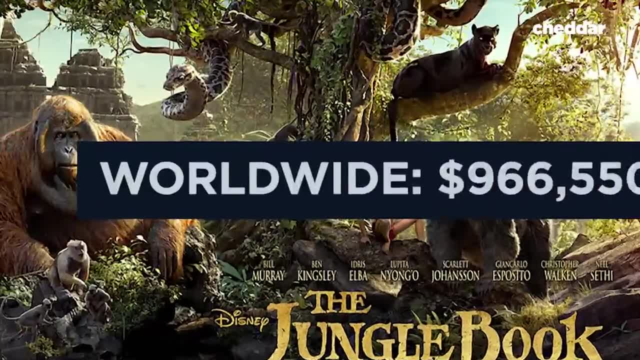 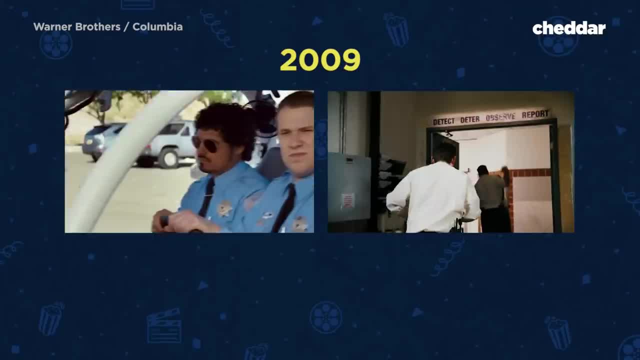 But it's a good thing they did, because The Jungle Book went on to make almost $1 billion at the box office, But it's not always so competitive in the world of Twin Films. In 2009,, there were two comedy Mall Cop films to hit the theaters: Observe and Report, and